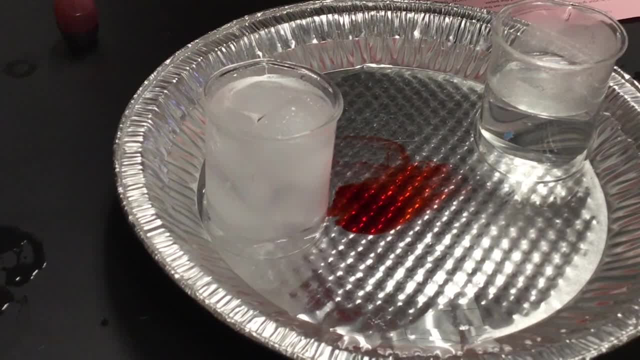 You're going to see little wispies rise, Wispies, Wispies. Oh yeah, I see, Oh yeah, I see. That's so fun Because warm water rises right, So it's warming up. 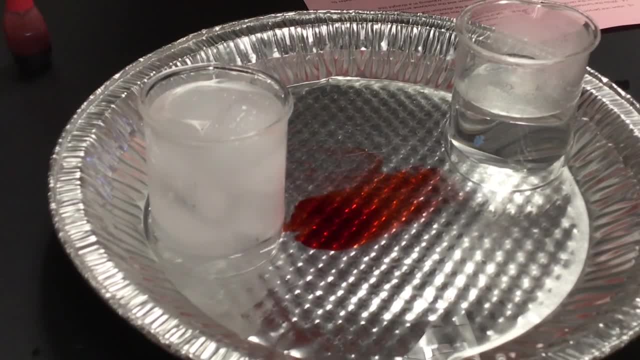 So that's your hot from the kettle And this is your ice water. That's your hot water from the kettle. Oh, I see it starting to rise. Do you see it against the beaker? It's rising, Yeah, Nice. 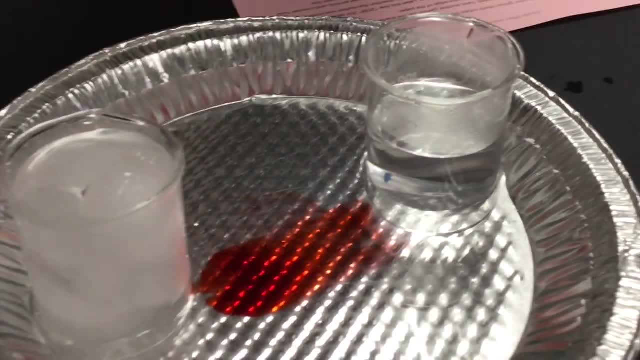 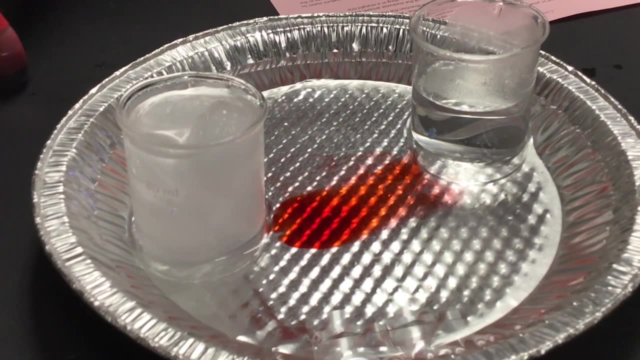 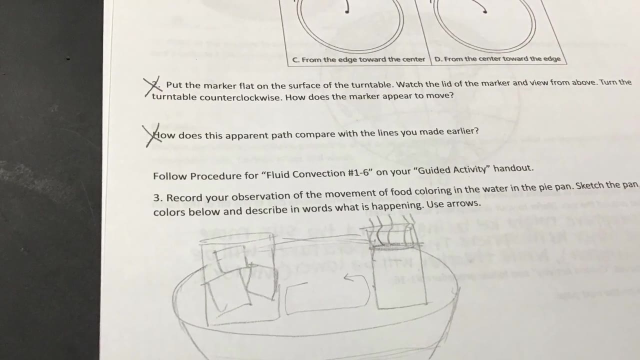 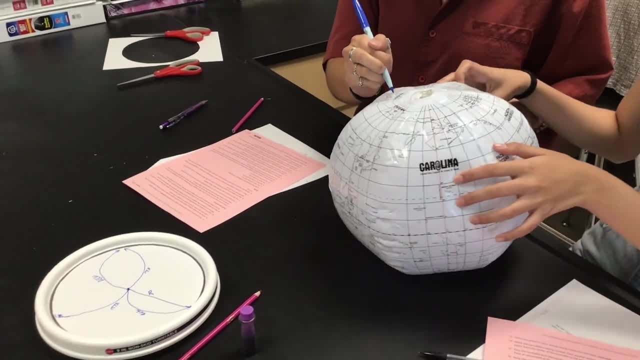 I love it. By the way, what's your mother doing on silver time? here, You see She's using some agolead yellow, She's using a sample of silver. Yes, This is a helps you actually see, Really, Yeah. 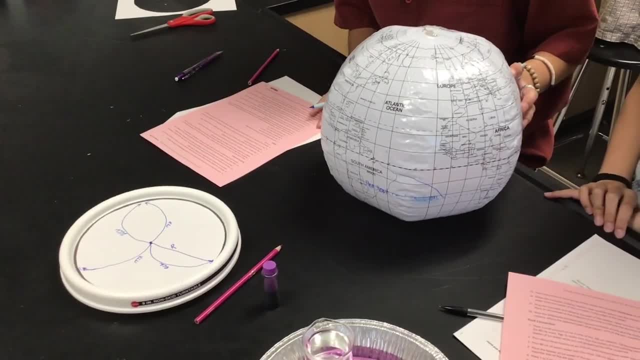 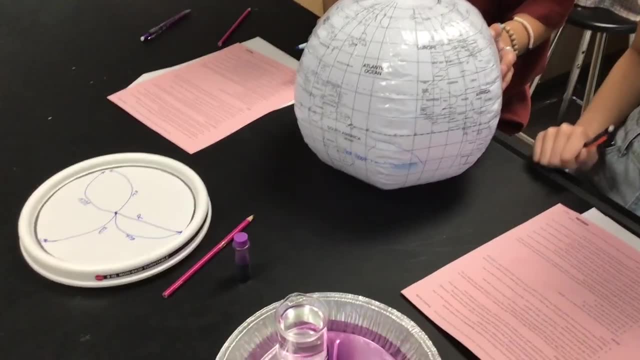 Yeah, You're not talking to her. Okay, Yeah, So let's see that line. Should I draw an arrow? All right, Very good, Thank you All the way down here. All right, So the next one, Kansas. 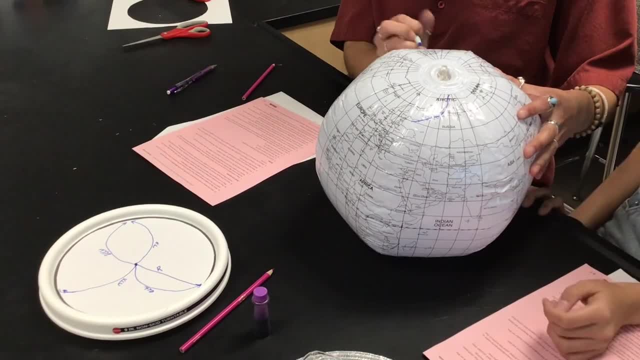 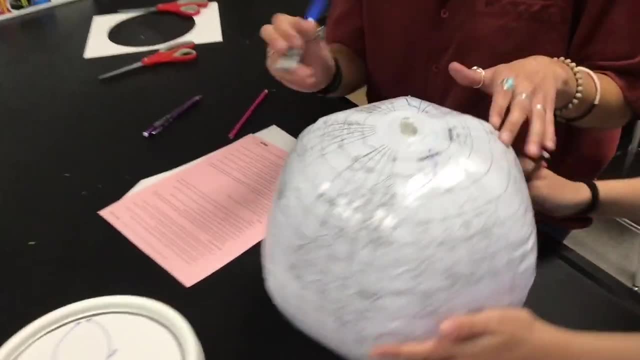 All right, I got to take it back, All right, and then turn it counterclockwise. All right, so turn it counterclockwise Good, All right, good, Let me see that line. It's not a very straight line. 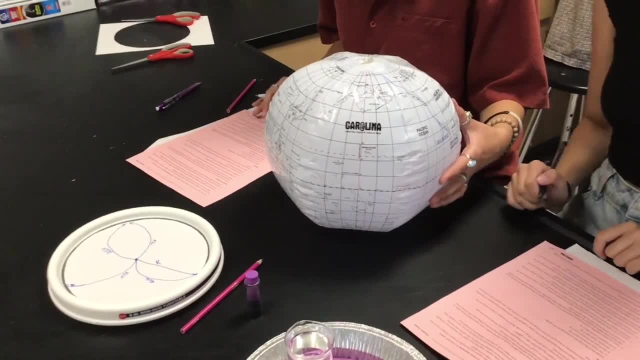 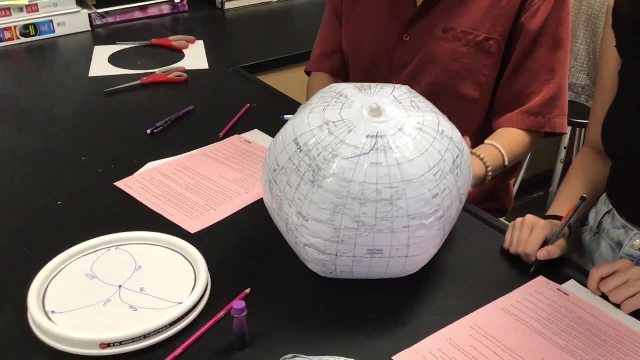 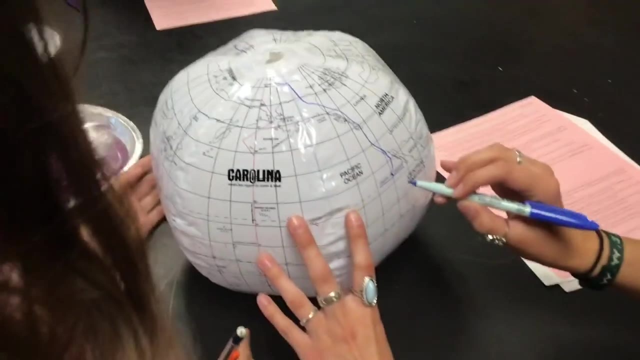 Kind of: Well, you can see the curve, Excellent, All right. And then from the top of the cancer to the equator, while we're going counterclockwise. Okay, wait, Let me do it from the same goal. This is for absent kids, okay. 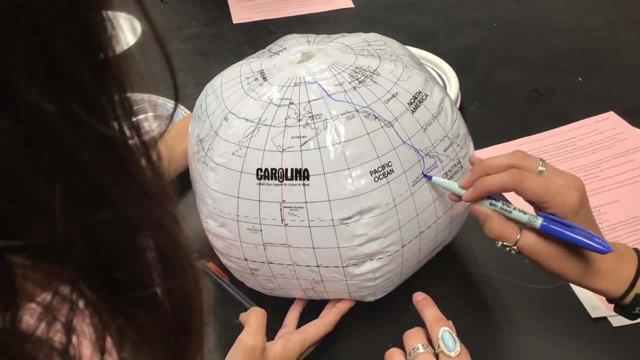 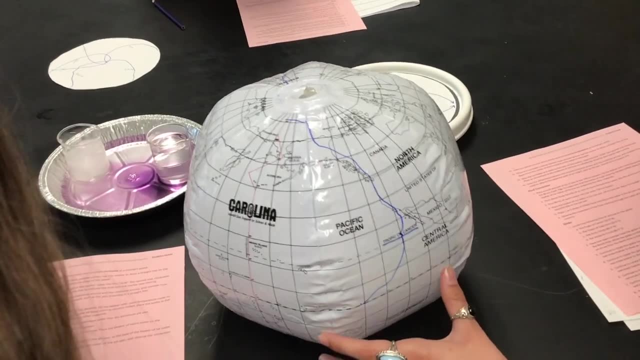 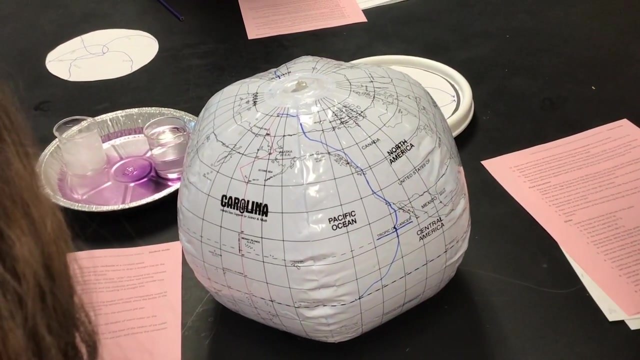 Wait, where did we put this? in the equator? Okay, All right, good. So let's see that curve. Nice, excellent, Okay, good. And then which one are we on Counterclockwise? Oh, that was topic of cancer. to the equator. 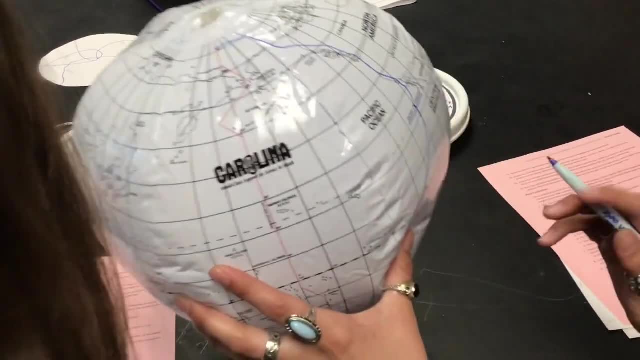 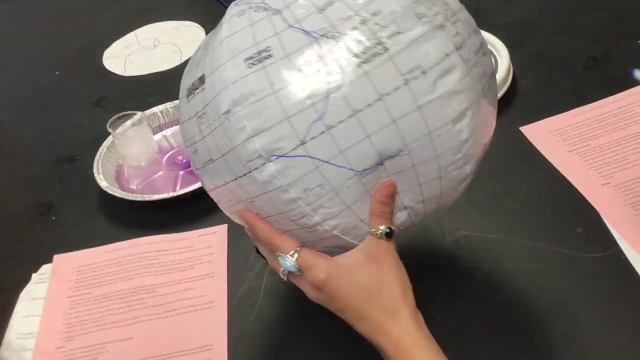 Now we're gonna do Capricorn to the equator, counterclockwise. still. Okay, you ready, Go ahead. And then Okay, All right. so let's see that. So you're seeing that it curves, depending on to the right or left. depending on where the location starts from, and whether it's in the northern or southern hemispheres. Here we go. Okay, so now Tropic of Capricorn to the Arctic Circle. Wait, isn't it the Antarctic Circle? Oh sorry. yeah, you're right.